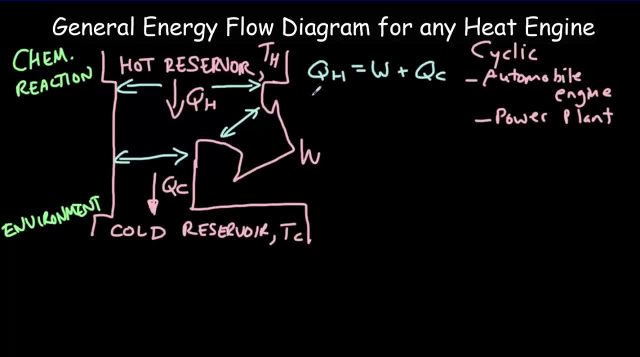 Exhaust heat QC, And I'm going to rearrange that. put the work on the left-hand side, So the work will equal QH minus QC. What we'd now like to do is write an expression for the efficiency. Now, I usually like to think of the efficiency as being the stuff that you want, divided by the stuff you've got to give up. 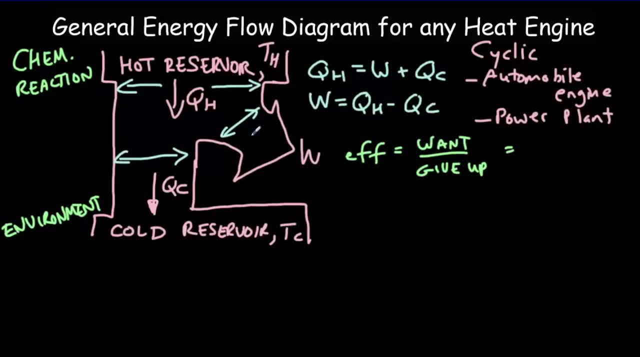 So in this particular case, what you want is the work. So in the power plant, the work is done, turning the turbines to produce electricity. In the car, the work is done pushing the pistons which makes the car move. So it's work divided by what you're giving up. 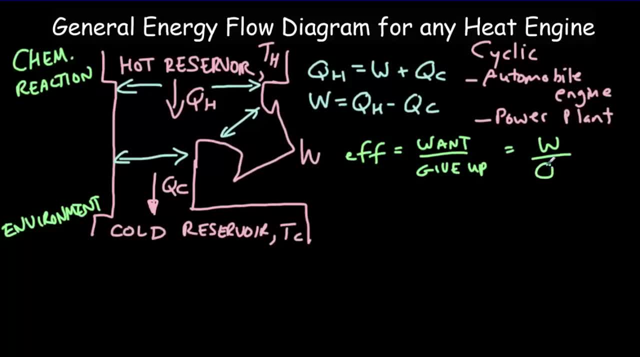 It's that heat coming out of the hot reservoir. Now the IB writes it a little differently. This is the expression out of your data booklet. They use the Greek letter eta for the efficiency. It's equal to the useful work done over the energy input. 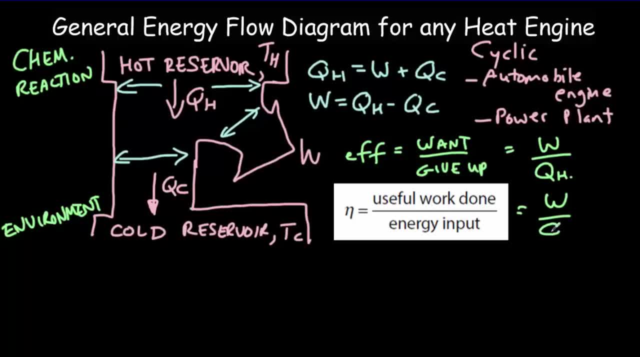 but it's still the same expression for our heat engine. It's work divided by QH. But what we can also do is use this expression here to rate our efficiency just in terms of the heat flows, so that we can rate that eta will be equal to Q hot minus Q cold. 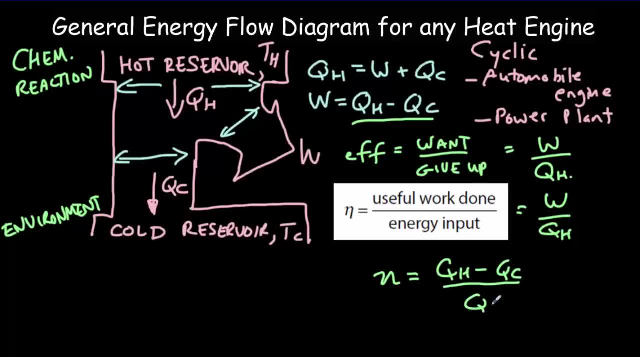 That's the work divided by QH, And often you'll see this written as 1 QH over QH, minus QC All over QH. Now we've got a general expression for the efficiency of any heat engine. And of course, the first question any engineer asks themselves is: 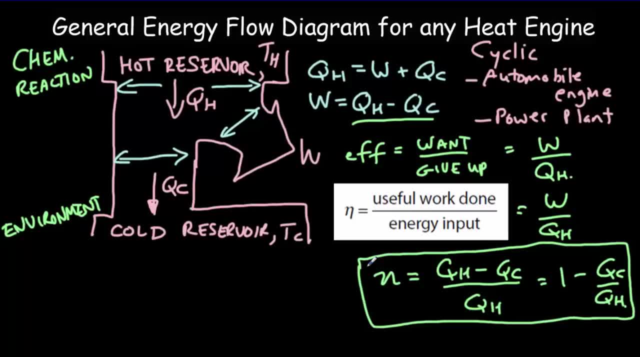 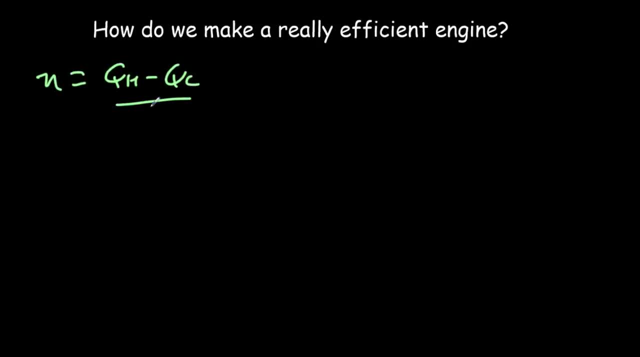 how can I improve the efficiency of the engine? So if our efficiency is equal to Q hot minus Q cold, all over Q hot, there's really not much we can do about changing the heat flow out of the hot reservoir. but what we'd like to be able to do is to reduce the heat flow into the cold reservoir or into the environment. 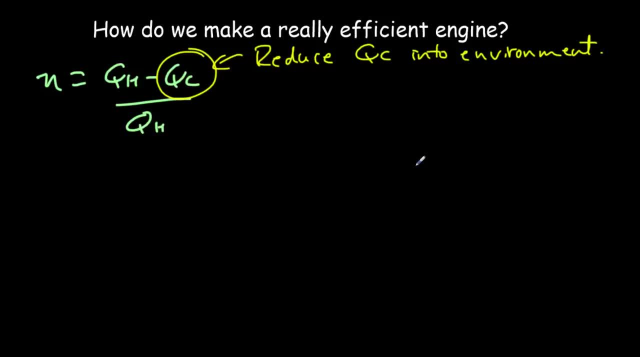 And we need to recognize there's really two sources to that heat flow into the environment. One of them we can do something about And one of them we can't do anything about. Now, where do our resources come from? Where's your pressure duplex? 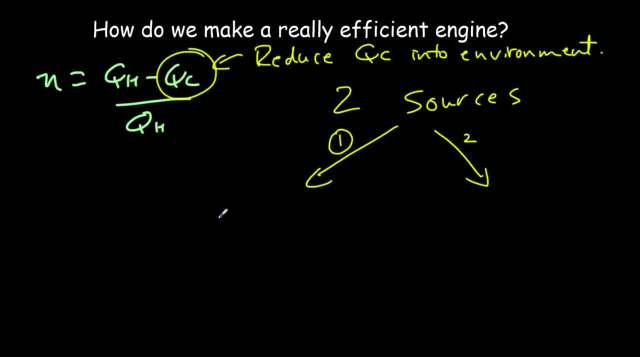 So Summer dividers are located in integrals right here on the right in quadrials. do anything about is basically where you reset your system. you have to exhaust the heat out of the piston so that you can compress the system and start the. 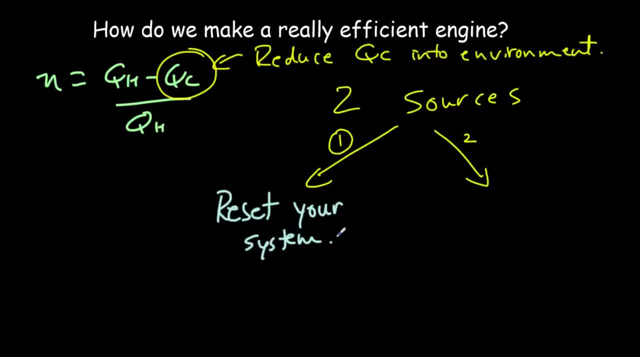 process again where you have to use a condenser on a power plant so that the pressure doesn't build up on the other side of the turbine and the turbine will keep rotating this whole process of resetting the system. you can't really do anything about that. the other source of heat flow into the environment is due to 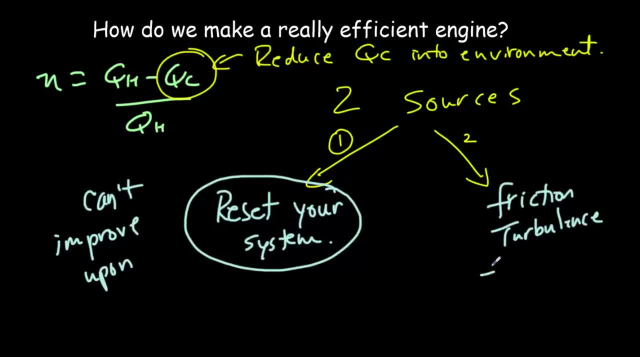 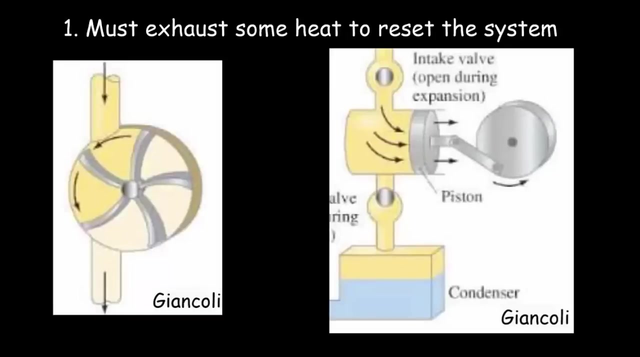 friction and turbulence. these are the things that increase entropy and cause the process to be irreversible. so the two sources are very, very important. let's take a little closer look at each of them. I've taken a few photos from Giancali to help explain this first source of. 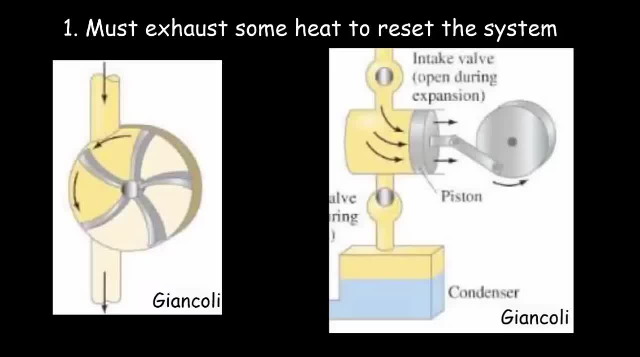 exhaust heat, which has to be used to reset the system. so we had said that no cyclic process can be a hundred percent efficient, and that's basically because we have to reset the system. so if, for instance, we have high-pressure steam coming into a turbine, that will only make 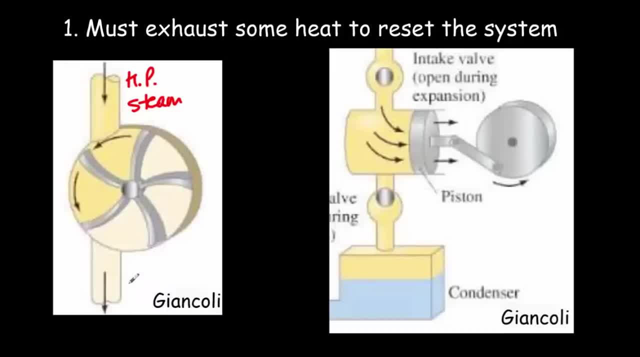 the turbine rotate around. if we don't have a buildup of high-pressure steam on this side, which means you're going to have to cool the steam on this side, use a condenser, say, and that means you're going to have this heat flow into the environment. that's your Q-cold. similarly, with this piston system, let's say we've 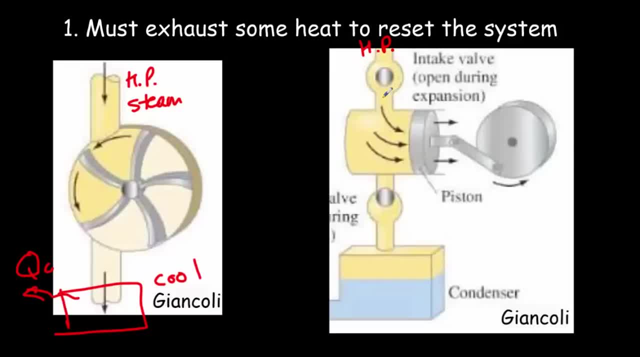 got high pressure here, this valve is open, but this valve is open and this is closed, and so that high-pressure steam is going to push the piston up and drives it up around this way and then it's going to come back again on the way back. this valve becomes closed and this valve becomes open and because we've got much, 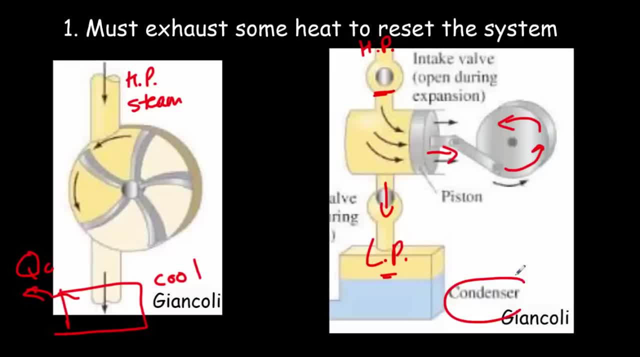 a lower pressure on this side. because we have cooling, because we have a condenser, because there is that exhaust heat into the environment, it's going to be much lower pressure as the piston comes down and that means you're going to have a net amount work, because when the gas does work it's high. 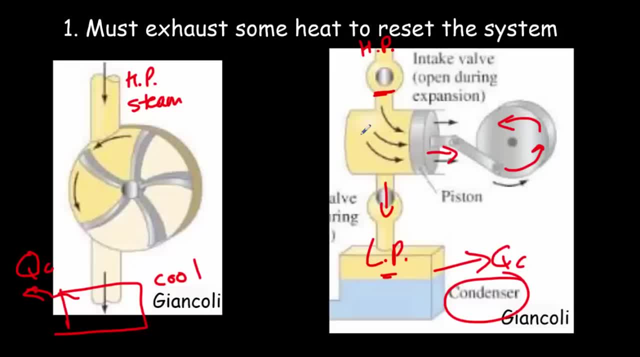 pressure, but when the environment does work on the gas, compressing it, it's at low pressure, and the net result is, of course, positive work being done. so in the end. when we originally made that statement that not all heat energy can be converted into work in a cyclic process, we were 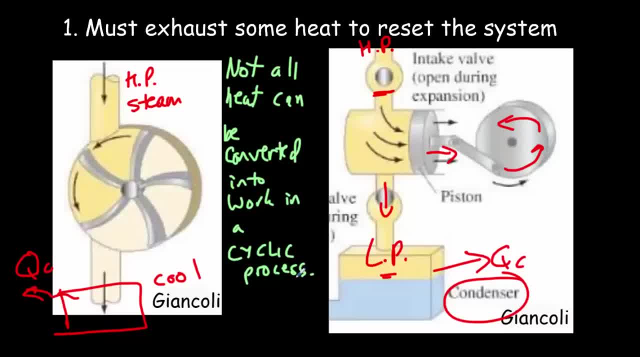 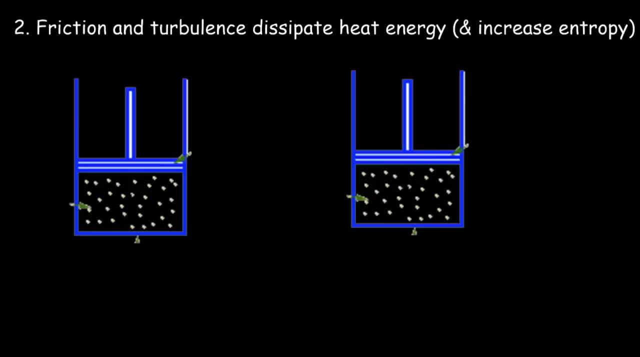 talking about the necessity of exhausting some heat in order to reset our system. so we can't really do anything about resetting the system. we have to reset the system. but we should be able to do something about friction and turbulence first. If there's friction, and that friction might be, say, the piston against the walls of 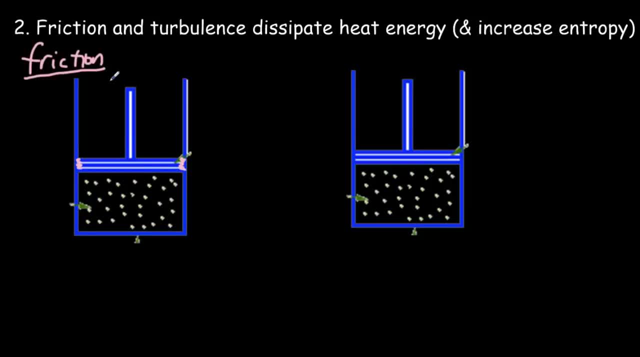 the container or this piston could be driving a crankshaft and there could be friction in the crankshaft. It could be anywhere in the system that there's friction, But of course, when there's friction and motion, heat is generated, and so you'd have some heat flow into the environment. 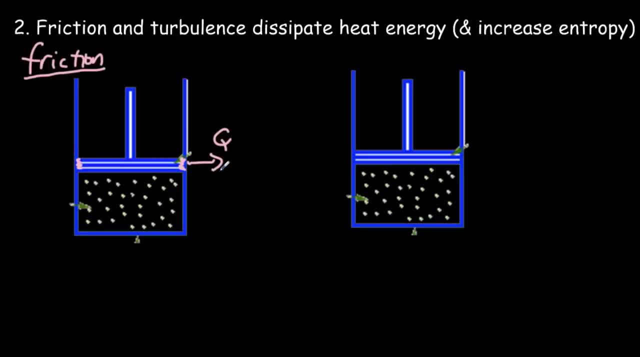 And that's going to make our system less efficient, naturally. And now let's consider turbulence, And maybe turbulence is probably too strong of a word. We could just say gas flow. So let's look at any sort of gas flow So you always get a gas flow when there's a difference. 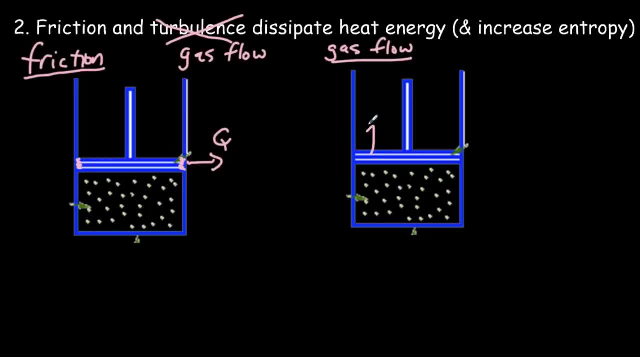 in pressure And let's say we just move our piston up quickly. If we do that, we're going to get a difference in pressure. There's going to be more pressure at the bottom of the container than there is near the wall of the piston And that means there's going to be a flow of gas. 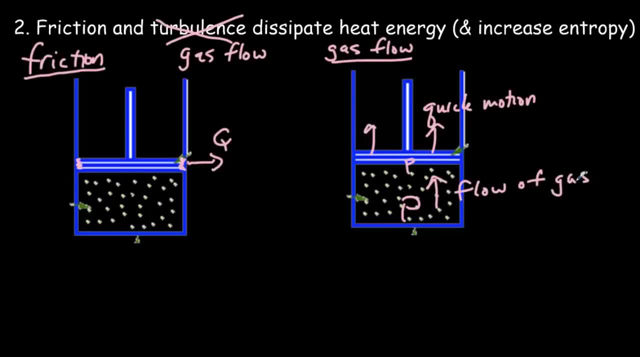 Well, whenever there's a flow of gas, you've got some friction there again And that means some heat energy is going to be produced and you're going to get heat flow. So once again, you're not going to be as efficient. Okay, let's try to get a little deeper look. 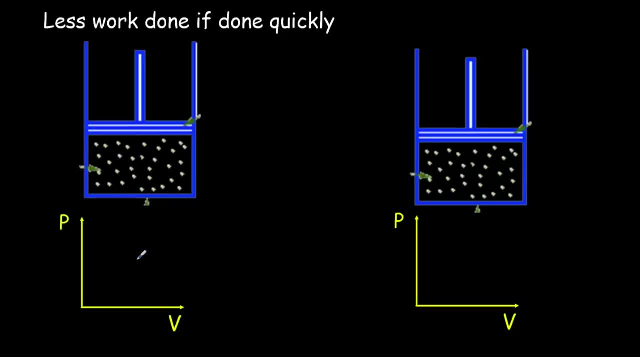 at this by considering a PV diagram for a gas going through an expansion at two different speeds. So the way we're going to get two different speeds is on this first gas we're going to place a large weight And that weight is going to contribute a pressure, And let's say that. 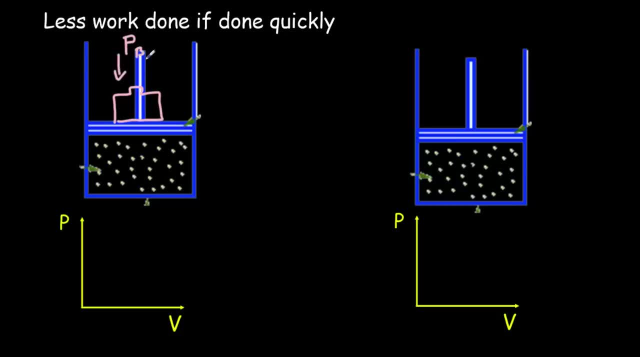 the pressure contributed is Pb for the big pressure, And so the total pressure would be atmospheric pressure plus that contribution due to the weight, P atmosphere plus P big. So that's our initial pressure and volume point, And then what we're going to do is: 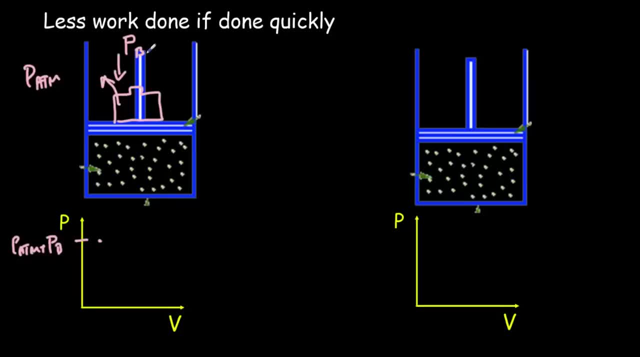 quickly lift the weight off so that the pressure immediately drops down to atmospheric pressure And the volume will increase. So let's say it increases to this volume here, but the pressure would have immediately dropped to P atmosphere. So the pressure was here at V1, drops down. 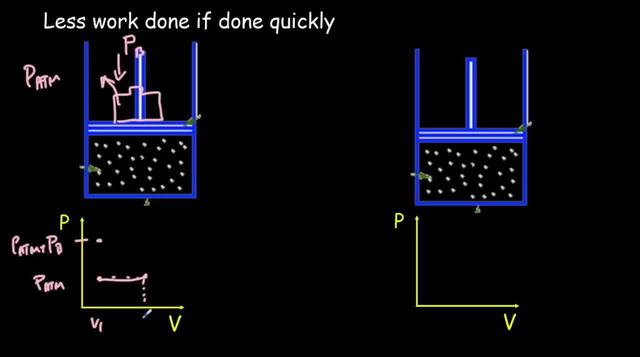 to here stays at that pressure P atmosphere until it gets to some other value V2.. And the work done would be this area. Now we're going to try the same thing, but this time we're going to put two equal masses. 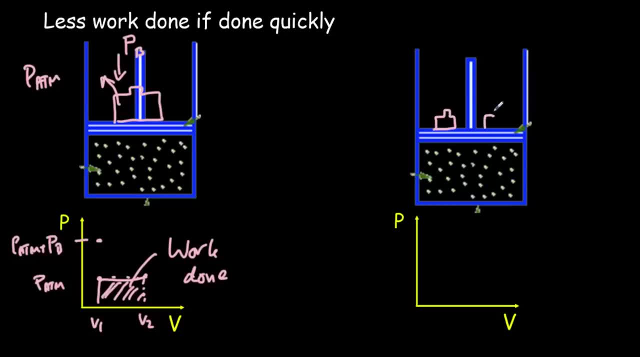 on here, each one half as big as our original mass on this side. So let's say the little mass contributes a pressure, P1, and the other little mass contributes the same pressure. So the total pressure would be the same as in the first case, It would be equal to P atmosphere. 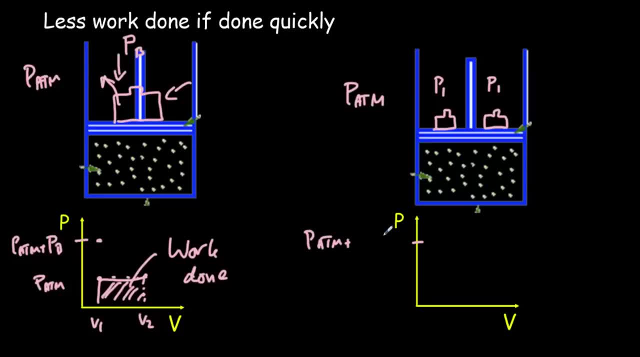 plus 2P1, or Pb, And there would be that initial volume, V1.. We're then going to remove one mass, then we're going to remove the other mass. Let's say, right here, we remove one mass, then the pressure is going to drop down to some value: P, atmosphere plus V1. And then 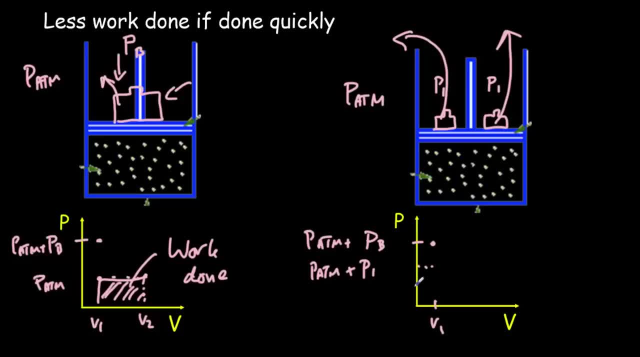 we're going to. sometime later we're going to drop the pressure down to just P atmosphere by removing that second weight. So our pressure started here, It immediately dropped down to here and then we removed the second weight and it dropped down to here. 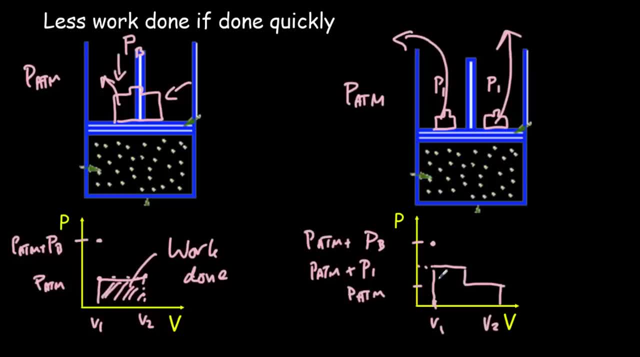 And we finished at the same volume. So you can see here that the work done is larger. when the expansion took place more slowly, when we did it in two steps- and of course, if we were to do this, say, one grain of sand at a time, we could get a. 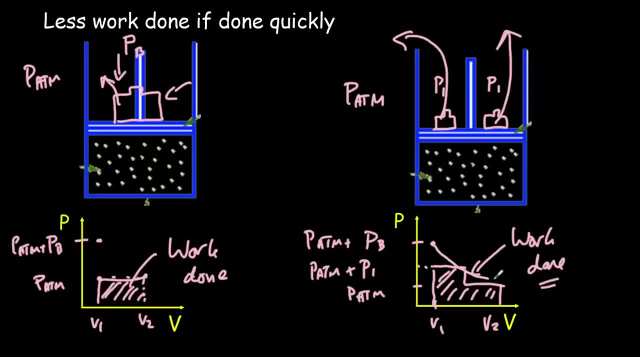 very smooth curve and then we would have a reversible process that's being carried out very, very slowly and our pressure wouldn't change suddenly. we'd have well-defined pressure the whole time. so, however you think of it, if we're going to have reversible processes where we're having sort of unnecessary heat, 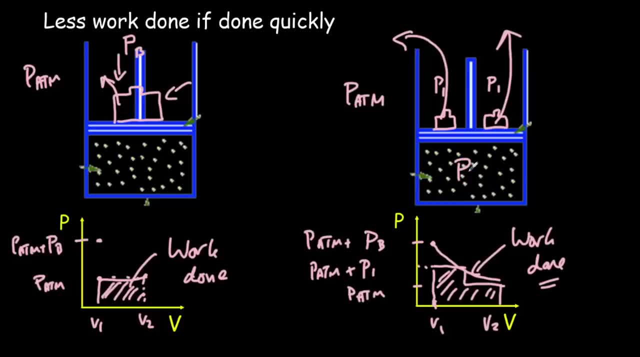 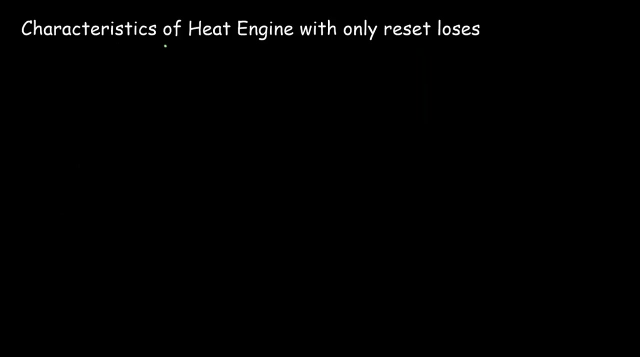 losses to the environment, then it's got to be carried out very slowly, effectively, so slowly that the pressure is consistent throughout the gas, and whatever the pressure of the gas equals will be equal to the pressure from the piston. so let's try to summarize the characteristics of a heat engine. 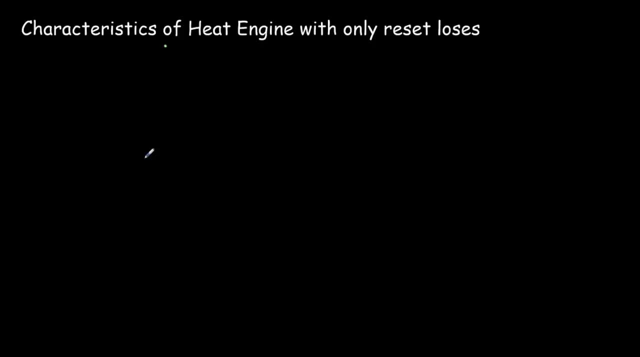 that we're going to have reversible processes where we're having sort of unnecessary heat losses to the environment, then it's got to be carried in. that only has these reset losses, and firstly, of course it's got to be no friction. secondly, there'd be no turbulence. but even more than that. 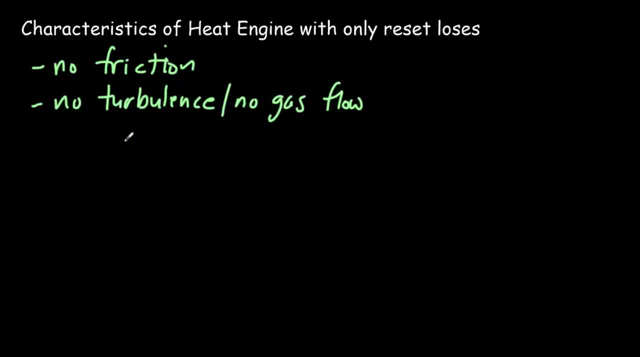 there'd be no flow within the gases. and if there's no gas flow, that means you've got consistent pressure throughout and that really implies you've got a consistent temperature throughout and you've got a consistent volume, meaning you don't have fuzzy edges to the gas. the gas is right up against the walls of the container and we can 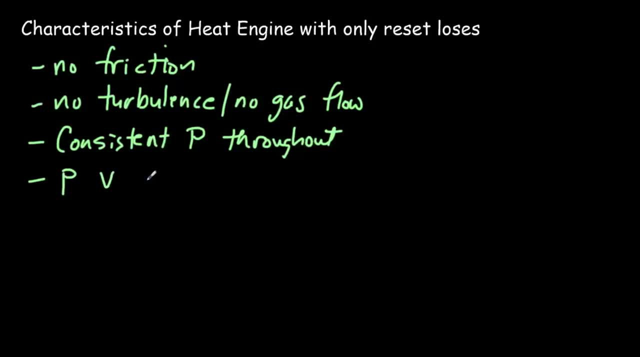 say that a couple different ways. we can say that P, V and T are well-defined. you might also hear the phrase that it's a quasi static process, which really means the same thing. the magnitude of the pressure of the gas on the piston has always got to be equal to the magnitude of the pressure of the piston and the 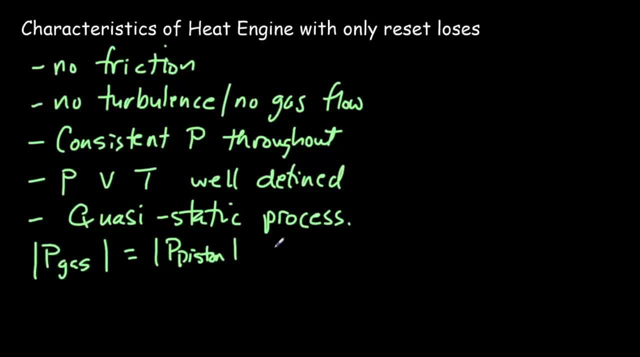 on the gas. in other words, you've got an equilibrium situation. now, in order to get this, it's the whole process is going to have to be carried out slowly, very slowly. usually you think of it as grain by grain and you can add the grains or subtract the grains to reverse the process. so it's got to be a reversible. 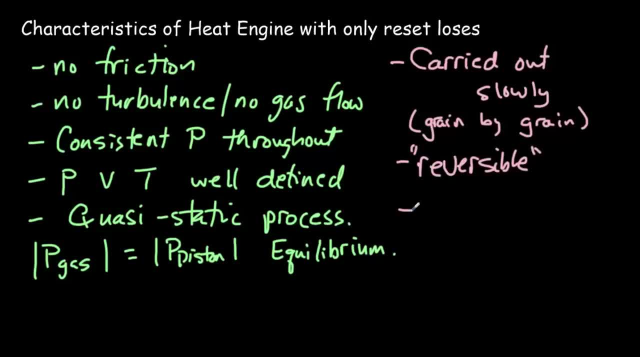 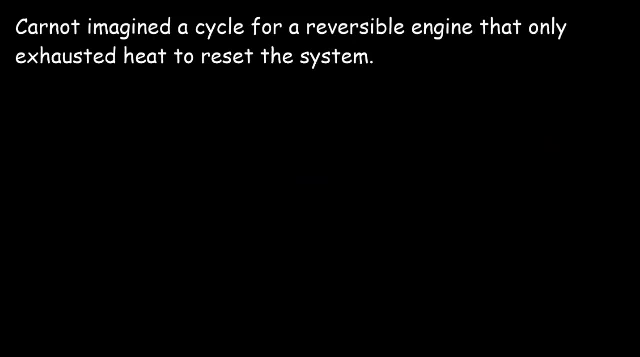 process and of course, for any reversible process. that means there's no increase in entropy to the gas over a complete cycle. in the 1820s, the grandfather of thermodynamics, Sadi Carnot, imagined a reversible engine, one that only exhaust heat to reset the system. now he's not really imagining how to build a reversible engine, he's just. 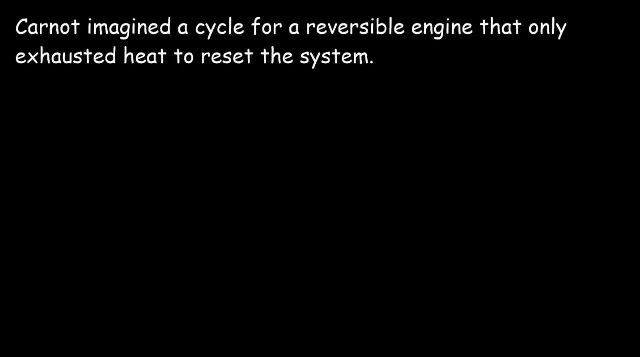 imagining a cyclic process that would be reversible and he wanted to pick one out. that's going to be very easy mathematically because there's some proofs that he'd like to do, and you'll recall from the video on PV diagrams that the Carnot cycle consisted of four branches there. 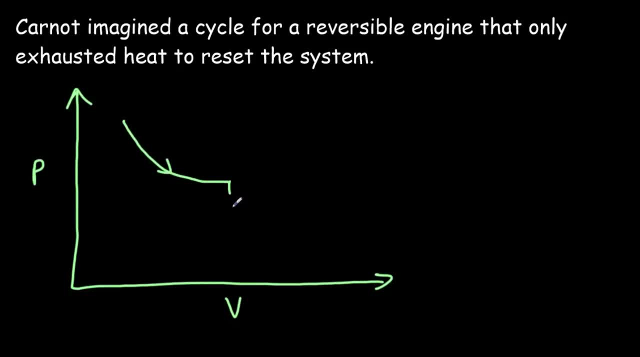 was an isothermal expansion, followed by an adiabatic expansion, followed by an isothermal compression and then an adiabatic compression. so it looks something like that now. of course, by definition the two adiabatic sections have to be reversible, because we know no heat flows to the environment during. 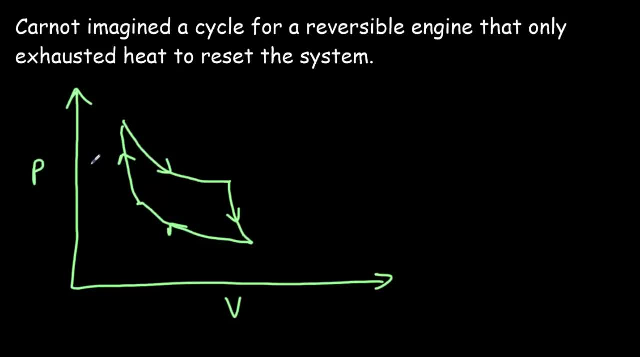 the adiabatic processes by definition. so here we've got Q equals zero. here we've got Q equals zero simply because they're adiabatic. now the isotherms: simply because you've got a well-defined temperature. you've got well-defined state variables. this is going to be reversible too. what really makes it? 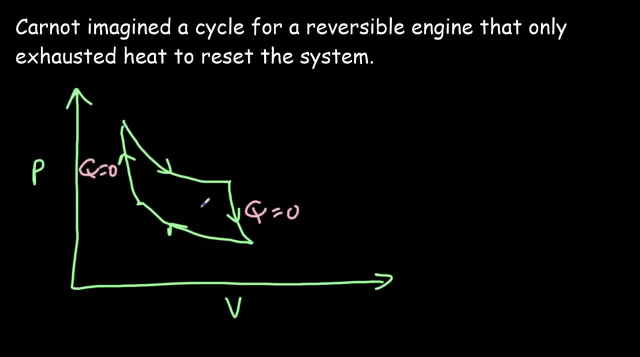 reversible is that it's going to be carried out slowly. so during this hot isotherm, that's where you place your gas on the hot reservoir and the gas absorbs some heat. that would be the QH. during the other isotherm, that's where you sit your gas on a cold reservoir and that's where the heat flows out into the. 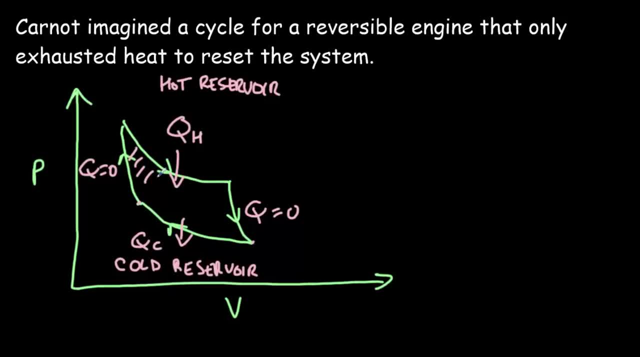 environment and of course, the work done would be this area in here. what Carnot showed was that that expression that we had for a general heat engine in terms of the heat flows, that one minus QC, all over QH, that's the general expression for efficiency. if you've got any reversible engine, then the equation for 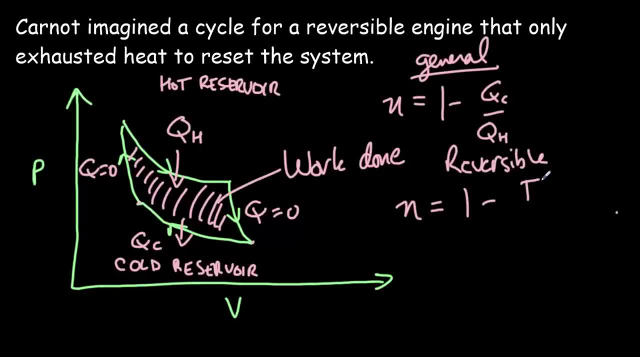 the efficiency looks almost the same, except that you can replace the amount of heat flow with the temperature of the reservoirs, so it will equal one minus the temperature of the cold reservoir and three minus the heat flow, with a long-term heat cold reservoir divided by the temperature of the hot reservoir and by 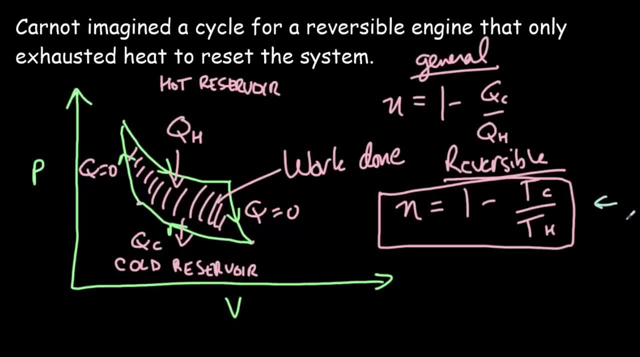 the way, this equation for the efficiency, it's not so difficult to prove with a bit of calculus. the primary thing that you'd have to be able to calculate is the work done over the cycle, and you do that by calculating the work done over each path, and you'll remember that work is equal to pressure times, the change in 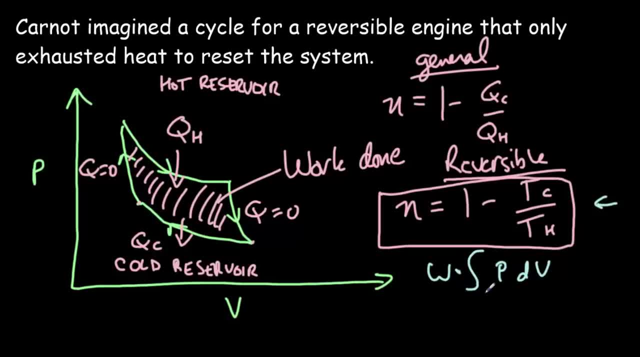 volume. of course pressure isn't constant, so you have to integrate over each part of the path P times Delta V. then we can use the ideal gas law to write that P equals nRT all over V and then at least along the isotherms nRT is constant. so 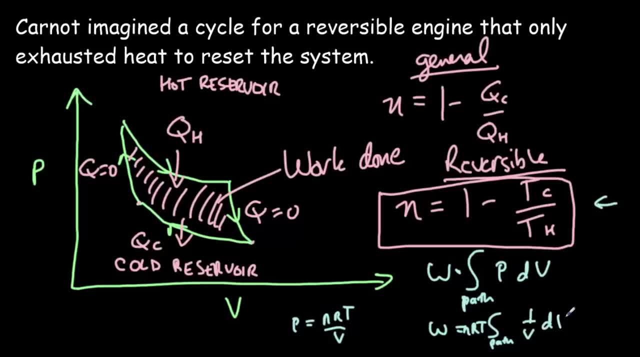 you're going to get a simple integral: 1 over V, Delta V over that segment of the path. I don't want to go into any more details, but I would like you to know that the proof, with a little bit of calculus, is well within our grasp. 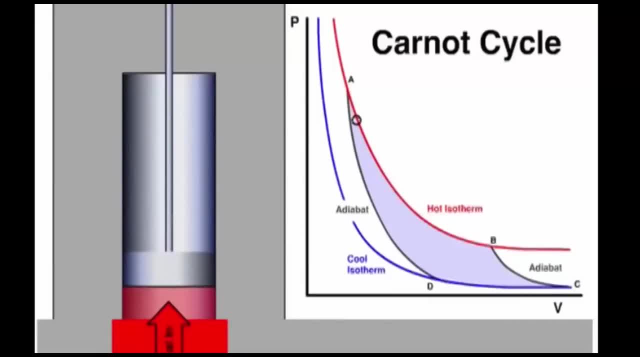 here's a good animation of the Carnot cycle. it's from Santa Barbara City College Science Department. right now it's on the isothermal curve. it's an expansion. grains of sand are being taken off the piston and the heat reservoir is providing heat to make it expand. it then switches to the out diabetic expansion. 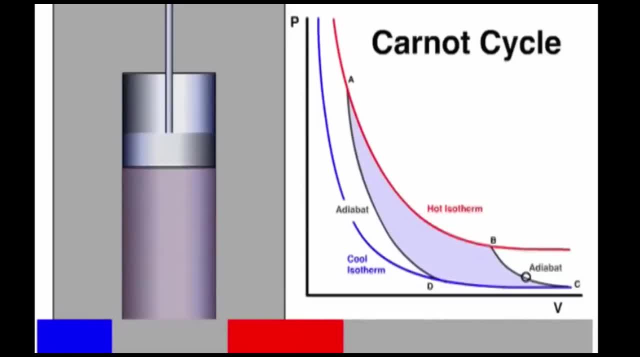 now. now the container is insulated, more grains of sand being taken off the top and that's why it continues to expand. until it gets to that point of maximum expansion at C switches back over to another isothermal curve. now it's compressing, grains of sand being added and heat is flowing out of the gas. 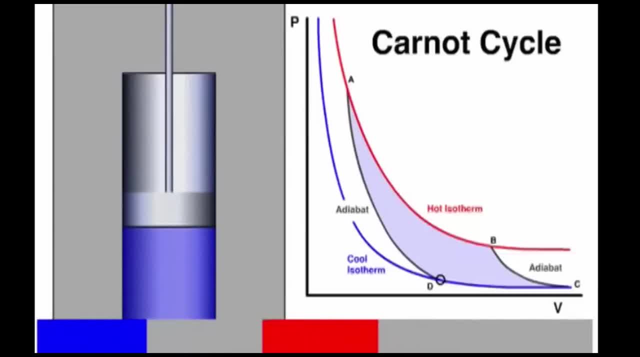 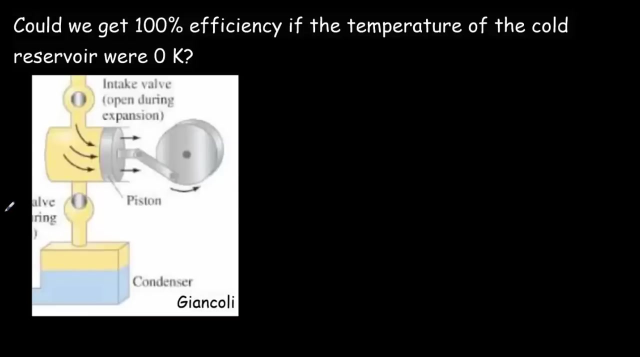 into the cold reservoir. it reaches point D, another I diabetic curve. no heat is going in or out, the containers insulated, more grains of sand being lifted off the piston and that's why it continues to compress until it gets to the point A where it's going to restart the cycle again if we take a little closer look at. 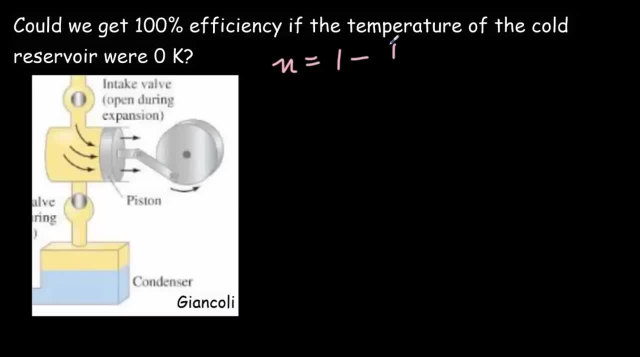 our equation for efficiency for the reversible engine, you'll notice that if TC were equal to zero Kelvin, then the efficiency would be equal to one. you'd have about 100% efficient engine. now it turns out through quantum mechanics it's not possible to reach zero Kelvin. 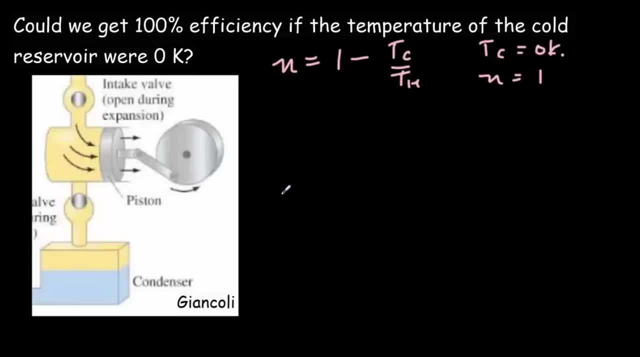 however, it's still kind of interesting to consider this possibility. so if our cold reservoir were at the zero K, then instead of having low pressure, you'd have zero pressure. so the high pressure comes in, pushes the piston up and then, when it comes down, this valve opens, this valve closes and the work is going to be. 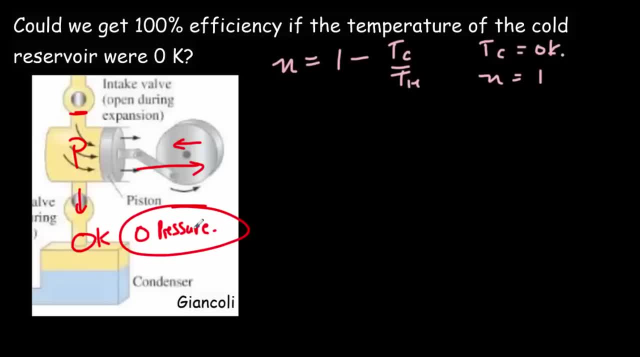 done against zero pressure. well, zero work is done against zero pressure, and that means you don't need to do any work to reset your system. and as a bit of a side point, this equation here would indicate that if it's colder outside, your car should be more efficient. 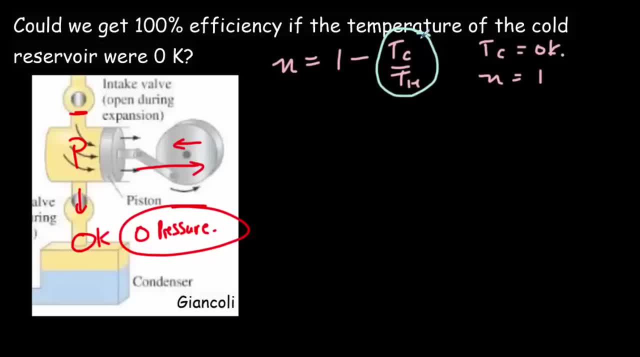 and that would be true if your car were a reversible engine. but of course there's all kinds of friction involved, and that frictions much higher in the wintertime when it's cold and the oil sticker and the oils are thicker. so it turns out your car is going to be quite a bit less efficient in the wintertime due to. 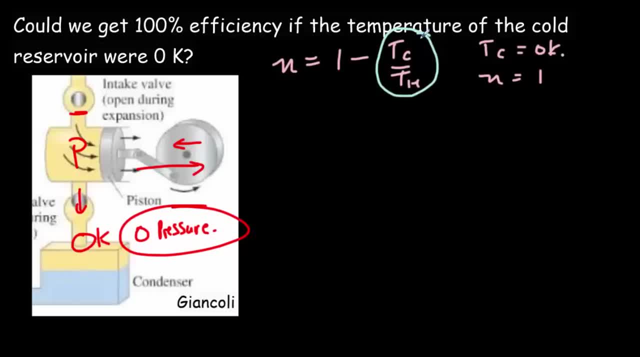 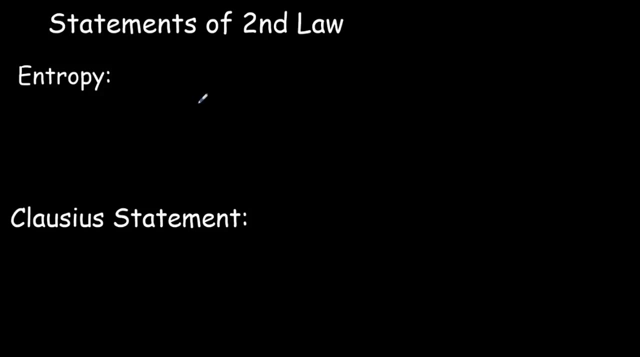 frictional effects, even though it's more efficient because less energy is required to reset the system for each cycle. in the video on entropy, I introduced the second law of thermodynamics and I said that the law expressed in terms of entropy was simply that the entropy of any closed system in 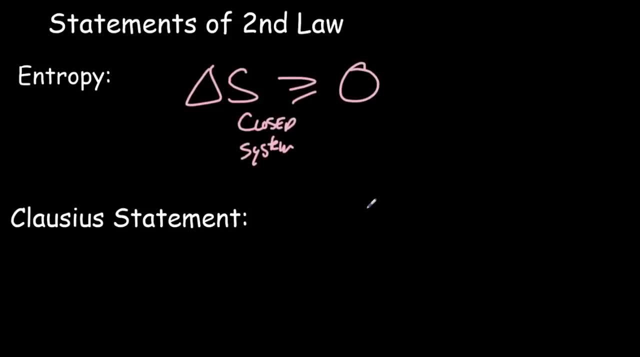 any natural process has to increase, and I also said that there were some other statements of the second law of thermodynamics. they were equivalent and we talk about them later. so these are the statements that you're responsible for with the IB. there's a Clausius statement which simply says that heat will not spontaneously flow. 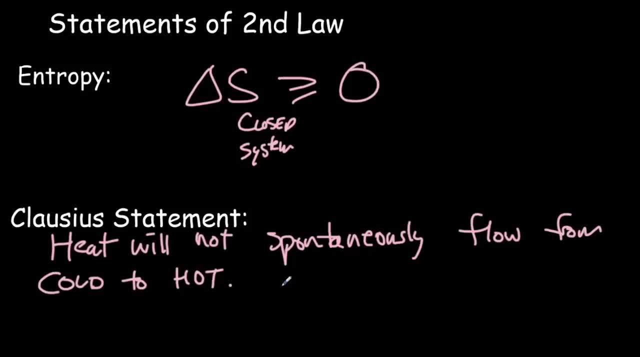 from cold to hot. you can get heat to flow from cold to hot, but you got to do work to make that happen. common examples of that include an air conditioner and a refrigerator. so if we've got two gases beside each other, one of them is hot, one of them is cold of. 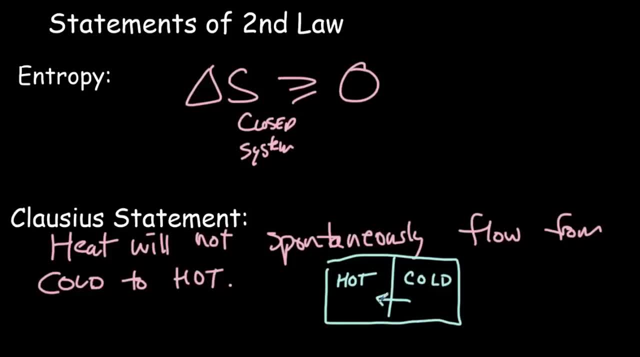 course, if heat flowed in the direction from cold to hot, the hot would get hotter and the cold would get colder. now that doesn't violate the law of conservation of energy- there's still just as much energy there. it violates the second law of thermodynamics, because if hot gets hotter and cold gets colder, 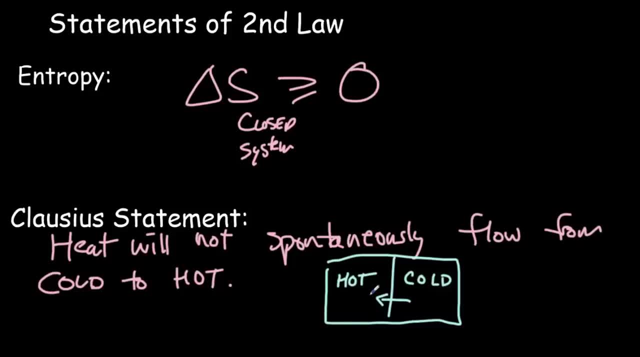 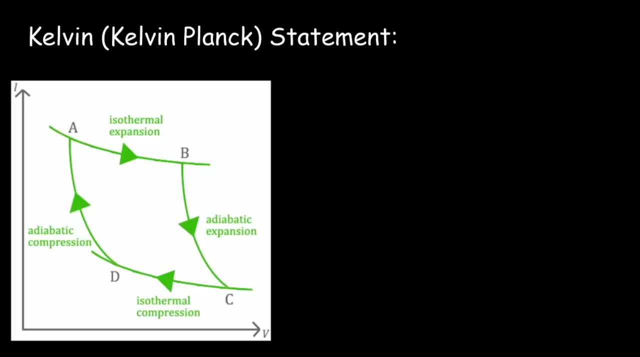 you've got a greater separation in temperature and if there's a greater separation, that's lowered entropy. so this statement is really simply a corollary of the second law stated in terms of entropy. let's now look at the Kelvin- or sometimes called the Kelvin Planck- statement of the second law and 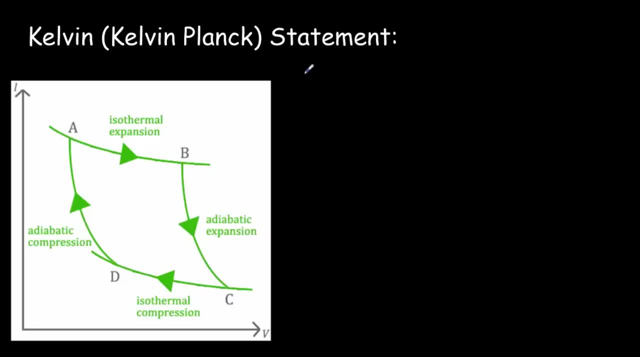 see how it relates to entropy increase. so the way it's usually worded is: a heat engine cannot convert all of the heat that's in the air into the air. so the way it's usually worded is a heat engine cannot convert all of the heat energy that it extracts into useful work. so we're really just saying: 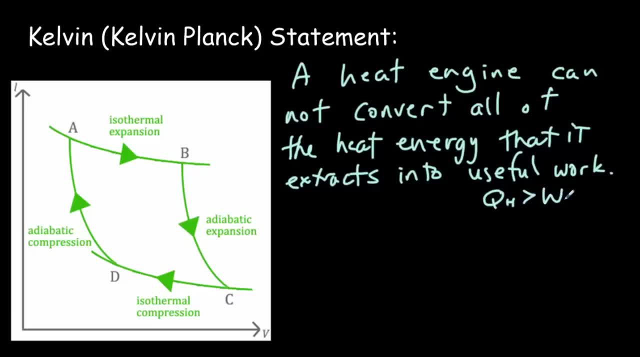 that that Q hot has got to be bigger than the work. so let's look at our best case scenario, the Carnot reversible engine, and see what happens to the entropy. and see what happens to the entropy along a cycle. so I'm going to give the entropy some arbitrary value at A. 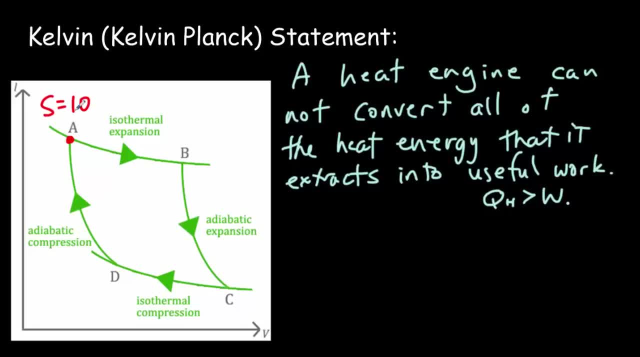 let's just say that the entropy at A is 10 units. now, during the isothermal expansion, at that hot temperature, the gas absorbs heat and hopefully you remember that the increase in entropy will equal to the amount of heat added divided by the temperature. so we're going to have a positive increase in. 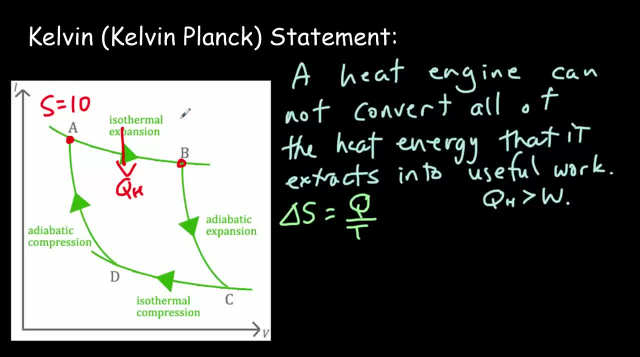 entropy as we get to B, let's say it increased to 12 units now during the adiabatic expansion. Q equals 0. that means you're not going to have any entropy change. it's going to stay at 12 units. when you get to C now. 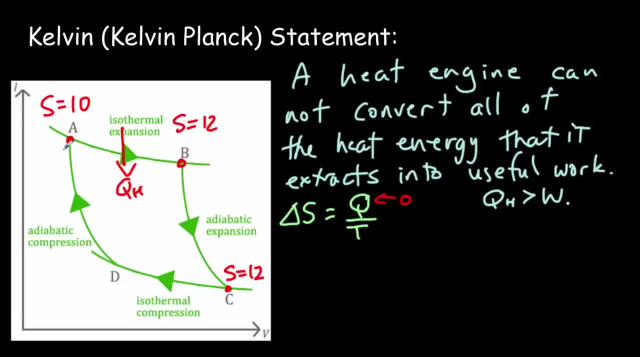 remember this whole cycle. it's reversible, so there can't be any change in the entropy over a whole cycle. so the entropy has to get back to 10 units. there's no entropy change along the adiabatic portion because Q equals 0, again P. so it's all got to happen along this isothermal portion. and how does it occur? 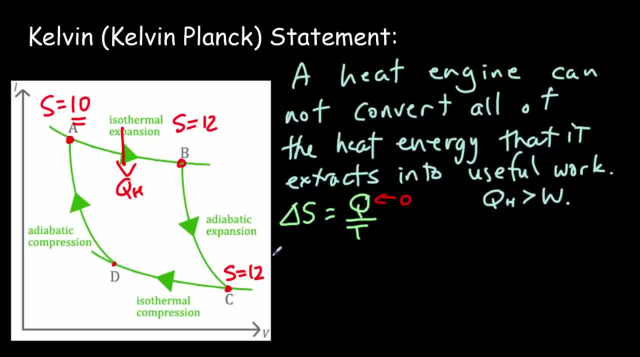 well, in order to lower entropy, we've got to release heat, that's that QC being released from the gas back into the environment. but remember, the temperature on this isotherm is less than the temperature on this isotherm and that means that we can get the same entropy change. 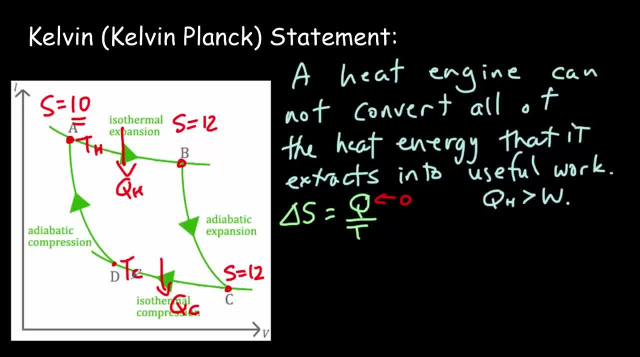 using less heat on the lower isotherm, which means that QH is going to be bigger in size than QC and our entropy is going to be down to 10 units once you get to point D. so, returning to our statement here, why is it that QH has to? 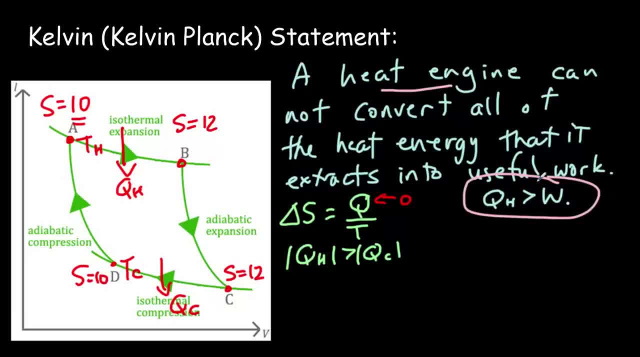 be bigger than the work done. it certainly wouldn't violate the first law of thermodynamics, the law of conservation of energy. however, it doesn't violate the second law of thermodynamics, the law of increasing entropy. that increase in entropy during the expansion needs to be flushed out, and that's done by releasing heat at a lower temperature, so that this